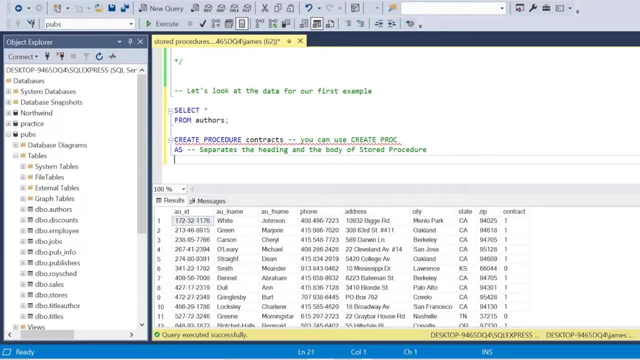 makes collaboration better as well. then we need to add the as keyword, which just separates the heading and the body of the stored procedure, and then- here you'll notice i'm going right to the end- we wrap um the sort of commands in between begin and end, and that's our basic syntax for for every. 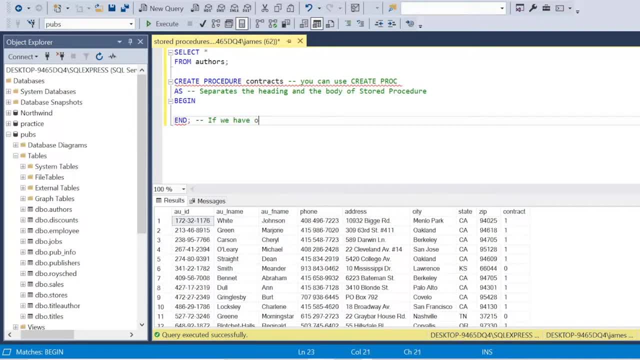 stored procedure and then we can basically use those queries or actions in between that begin and end. i have stressed here: if we have one statement, the beginning and end keywords are optional. however, i'm going to keep them again. it's the same as the the longer keywords. here i'd rather 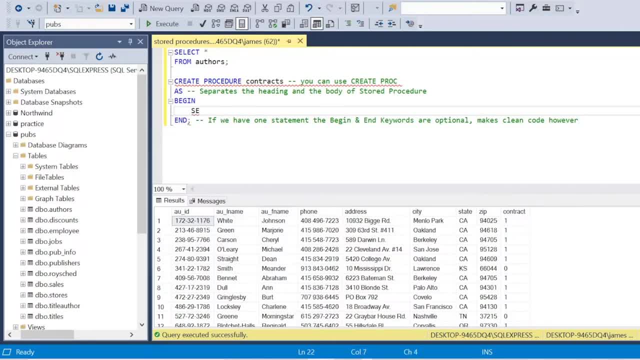 have some clean code. so i just have a little indent, and now we're actually going to look at how we can create a reusable procedure. so i'm going to select the state column and i'm just going to count contracts. so basically i want to see the amount of contracts by state. could be an. 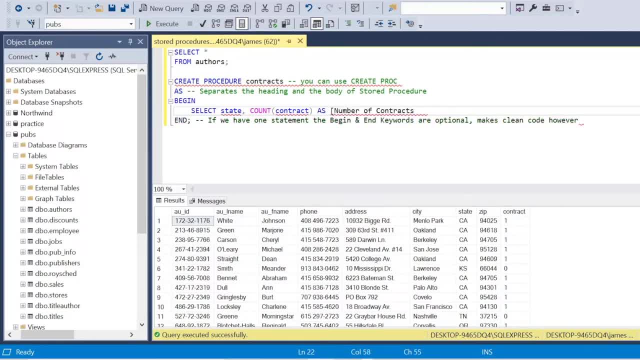 everyday task, or we could do this every every few months. so it's reusable. i'm going to call it. use an alias: number of contracts that count of contract column. remember, if you want to include spaces in your new column names, you can just use the square brackets. it's from authors and i want to group. 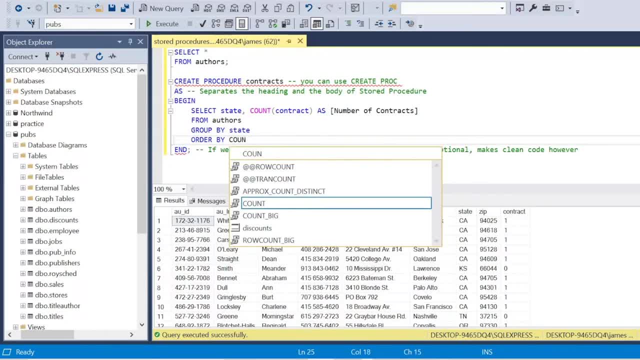 this by the state so that i see the level of contracts by state, that granularity or aggregation, and i'm going to order it by the count of the contract and i'm going to say in descending order, from highest to lowest to lowest'm going to say that i want to group this by the state, so i'm 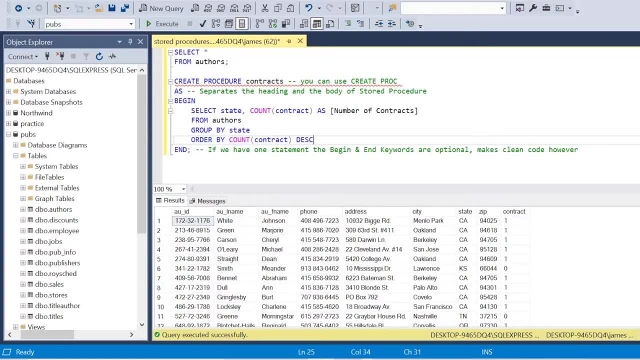 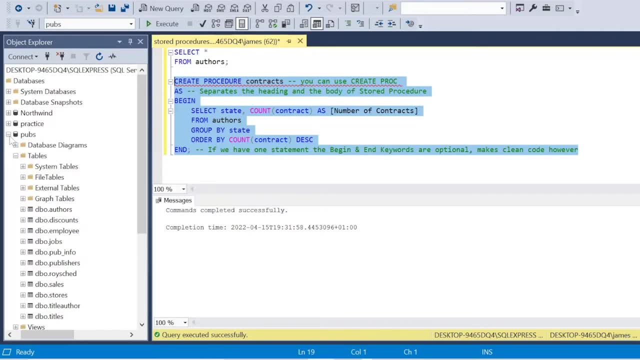 lowest. so we have a normal SQL query. there's nothing extremely complex here. but when I click execute it tells me that is now a stored procedure, essentially. so when I refresh the object explorer, go into programmability and stored procedures, you can see it's there in contracts. so how do we? 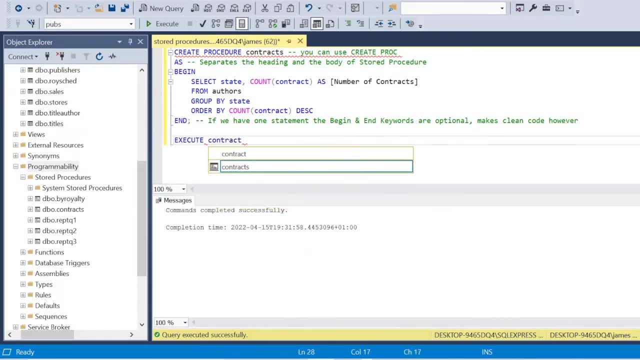 actually call this and get the results. well, we can use the execute keyword and the name of the stored procedure and you'll see that appears in our results. so execute contracts. again I'm going to say here in the comments you may see people just use exec again. you can do that, but again, 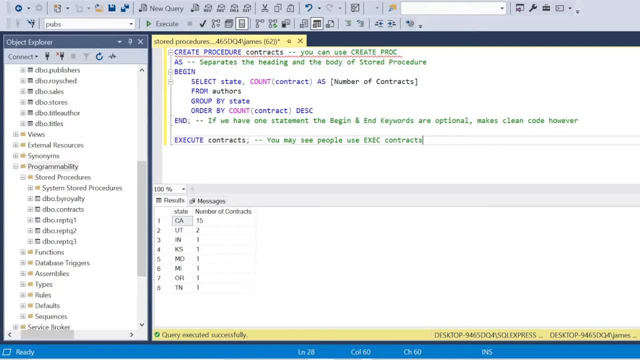 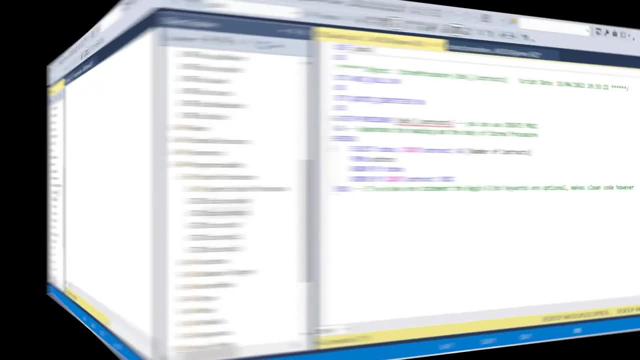 we'll just focus on specificity and clean code and I probably wouldn't change this anyway. I'd like to type it out in full so that I know when we work collaboratively everyone's on the same page. so if you go to the object explorer, actually right click in your stored procedure itself. 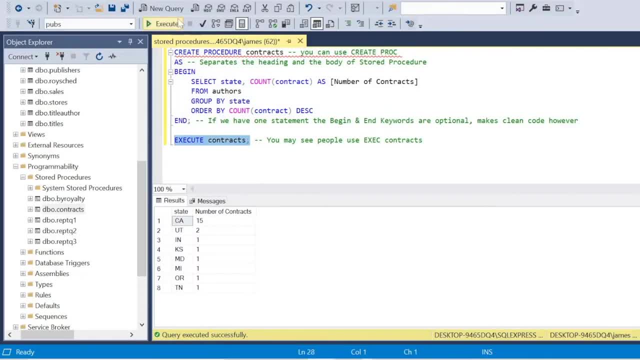 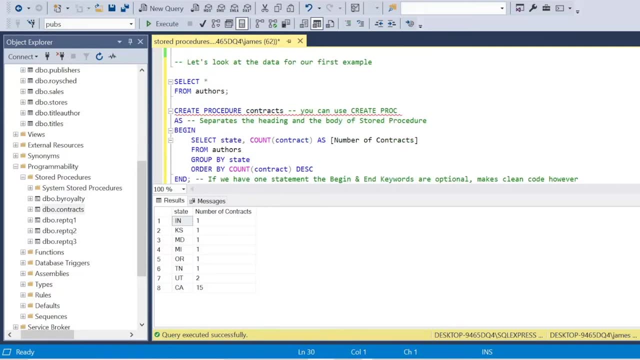 you can change it, you can modify it. so what I've done is I've actually just taken away descending, so the values show low to high in the default ascending order. so that's how easy it is to modify a stored procedure. now, if I want to delete a stored 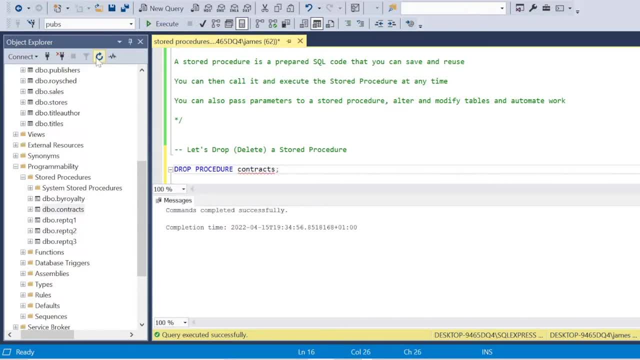 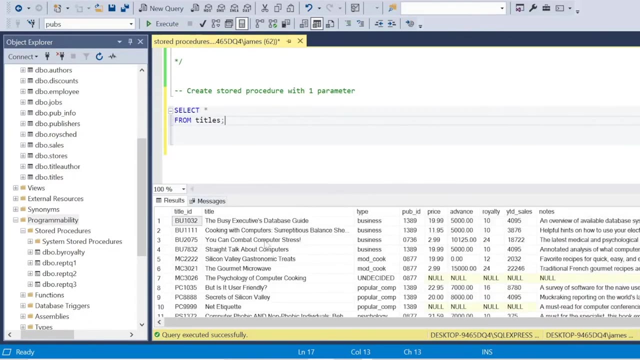 procedure and we call it drop. I can just select type, drop procedure and the name, and there we go. if we go back into our object explorer programmability, it's now gone. so let's look at how we can create a stored procedure with a parameter. so let's make. 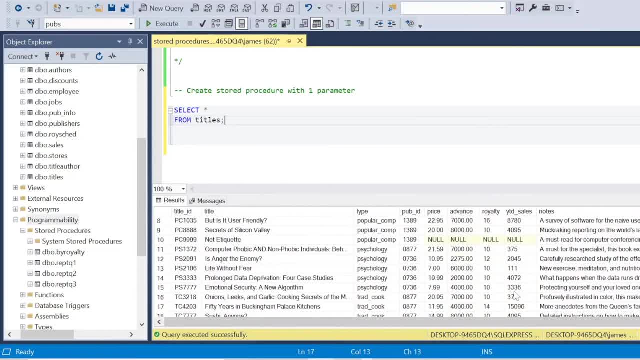 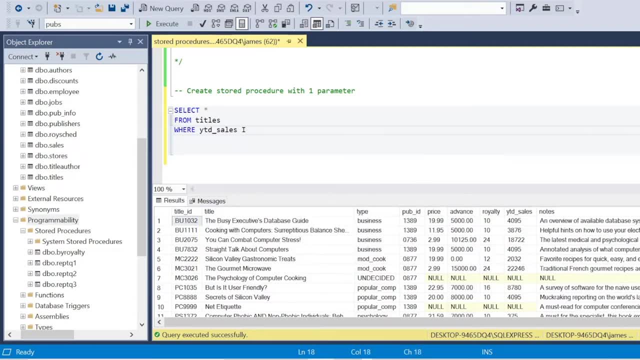 this dynamic and you'll see an issue here. when I select the details from titles, select everything, you'll see the year to date sales column has a nulls. so I can actually say just in this basic query where year to date sales is not null. so I want to filter those out and we're going to carry. 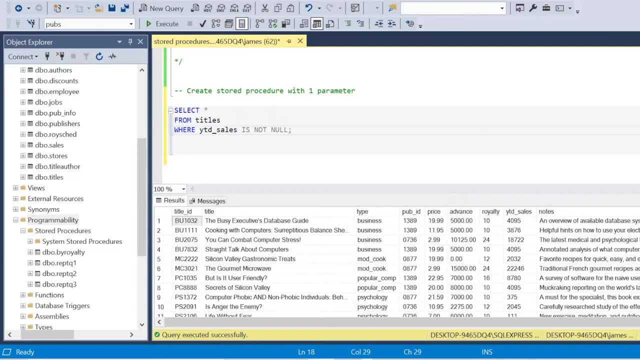 that through to our stored procedure with that user input, that parameter. so we make this even more valuable. and this is where store procedures sort of kick up a gear. so again, basic syntax. I want to create a procedure and I'm going to call it title sales, so sales of the year to date, sales of a title. but here I'm going to use at and I'm 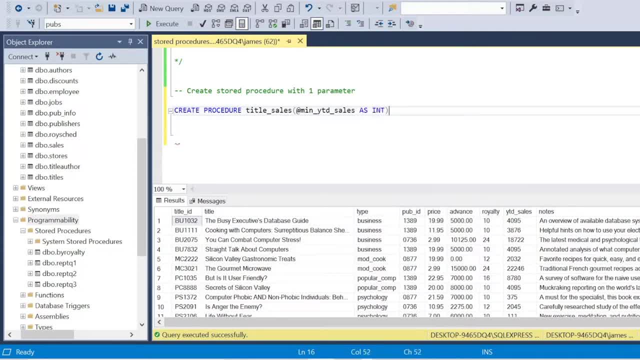 going to call this minimum year today. today, sales is what we're going to use as our parameter and it's an in, it's a whole number, so you give the data type as well. I say as and begin. we've looked at that before and I'll go in and do what we want to do with this query, so select. I want to select. 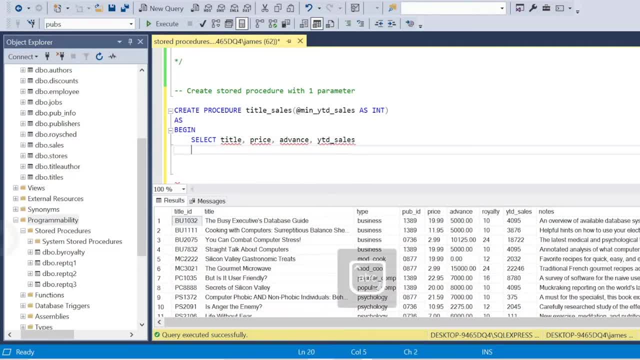 the title, the price, the advance, because that may be important to a year to date sales. we might want a correlation later from the titles. so it's from within the the titles table, but here I'm going to list two conditions. so I want where the year to date sales is greater than or equal to the 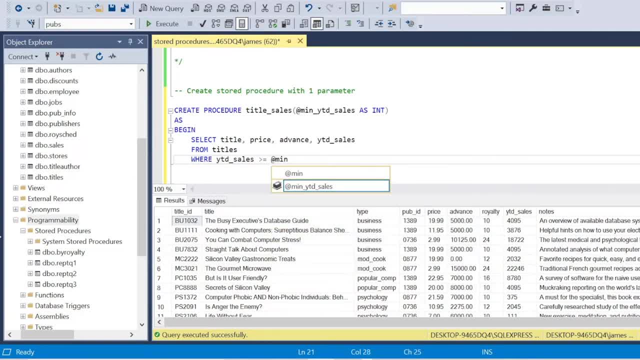 parameter that the user enters at the very start. so you see that admin underscore y, ytd underscore sales, and remember what we said: I want to ensure that the year to date sales is not null. I don't know. so let's say in this case, I don't trust that data, that underlying data there may be issues at. 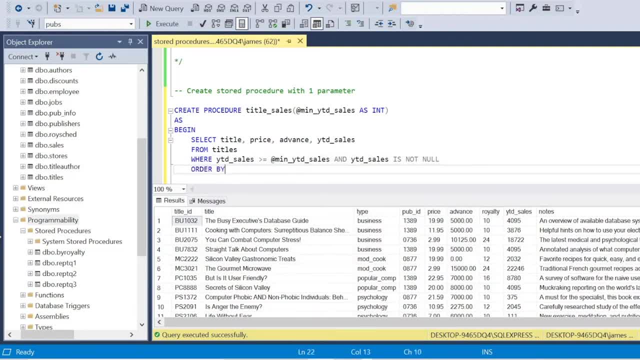 source. so I'll leave that out and then I can say I just want to order by the year-to-date sales in descending order and then end, and we're going to see how the user can enter a parameter and we can make this dynamic for for everyone involved or for us, if we're just analyzing different depths. 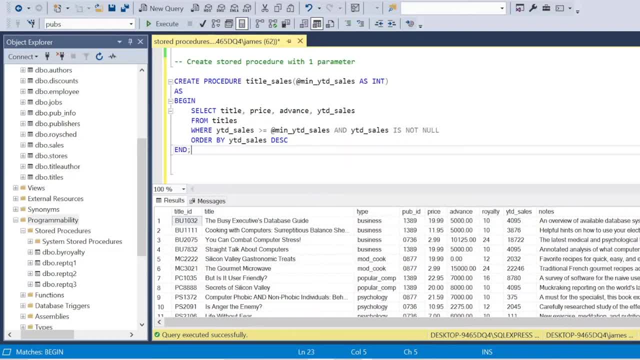 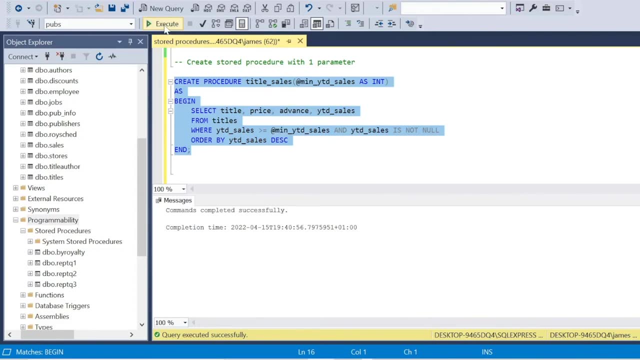 of data. so sticking to the syntax. but now that at value where the user can enter a parameter, will execute this and this will now become a stored procedure again within our object Explorer. so how do we call this? how do we use this? how do we make this functional? because obviously we've got this extra parameter. well, now, actually, all we have to 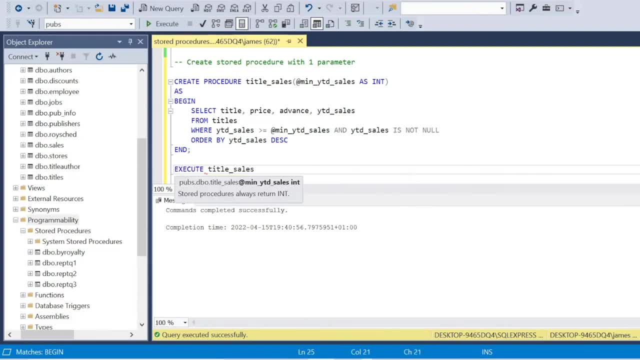 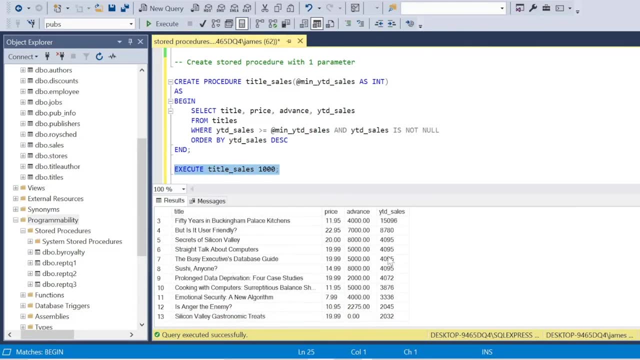 do is, again, we can use the execute and we're going to execute title sales. the name is store procedure, but you can see here at the end I put my parameter. so I want sales greater than one thousand or equal to or greater. now I put 10 000 and the data dynamically changes with that query. it's reusable. 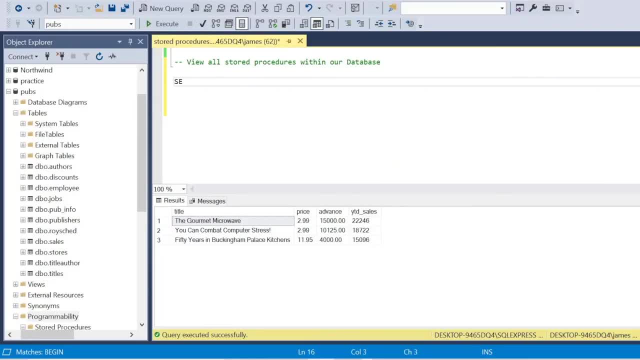 it's fast. so, yeah, great use case. now, if I want to view all the store procedures within our database, or if I was in master within any database that I have access to or I've created, all I need to type is select schema name, scheme ID. you can just use this verbatim as it is and I'll indent that with. 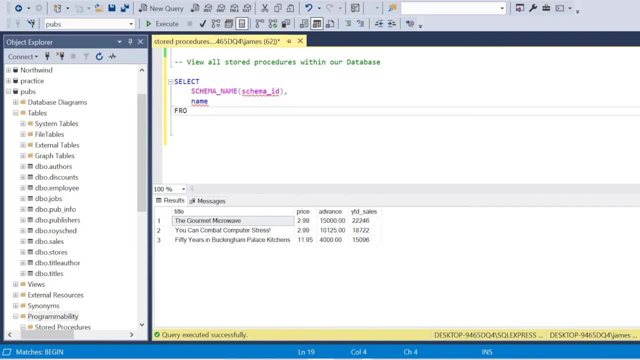 name on the next line and then we can just say from is dot procedures and where the type is equal to P, because this will just return the sort of default stored procedures if you specify P, and there we go, we can see all of the store procedures we have. 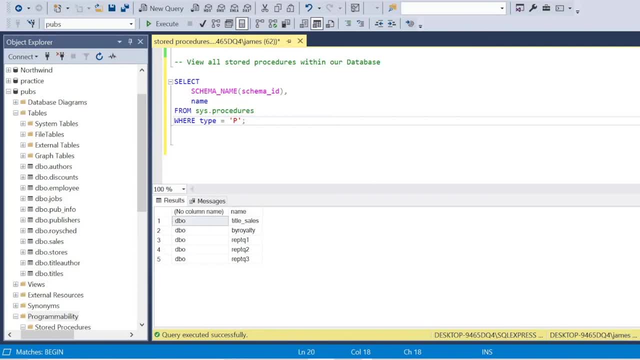 and you can see our title sales. we won't see contracts because we deleted that and dropped it, so everything works well. well, not a lot of time but, I hope, a lot of great content and, as usual, if you like this content, please feel free to like, comment, subscribe and share. thank you.